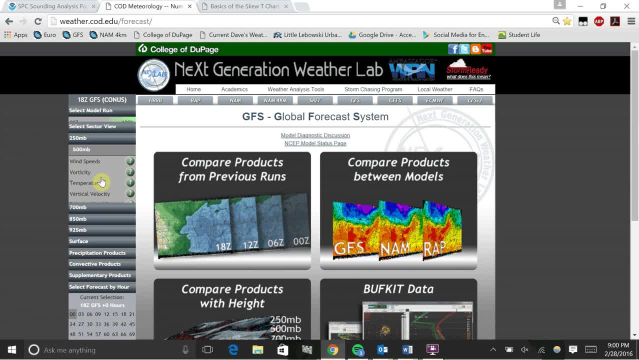 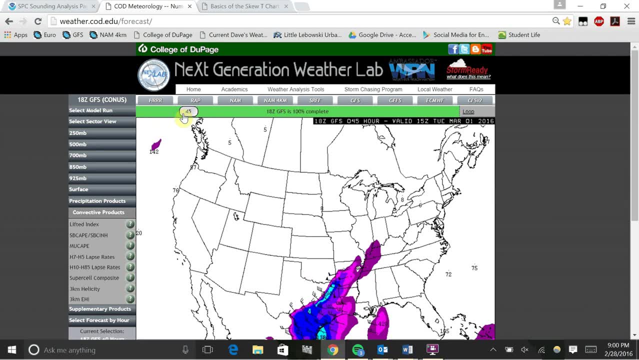 Really any model is going to give you good SCU-T data, So let's go down. Let's just choose some convective parameter here, See if we can get some CAPE going. We'll talk about CAPE a little bit later. 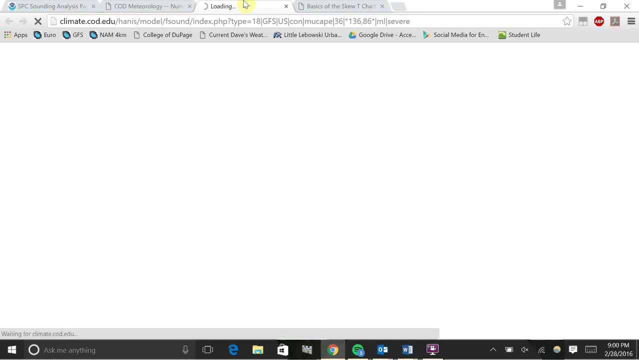 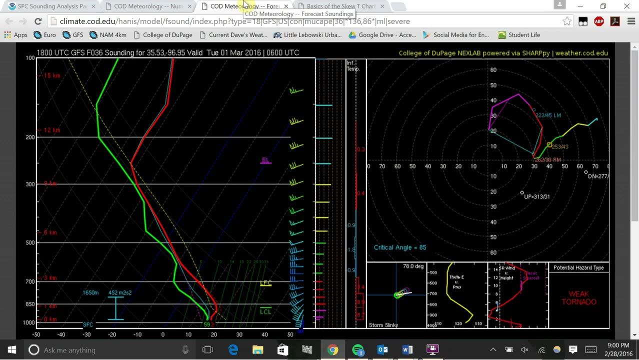 So I'm going to click here and it's going to take a second to load. They're actually switching to some new software that's developed here at OU, So they're trying to work out some kinks, but it still takes a little bit. 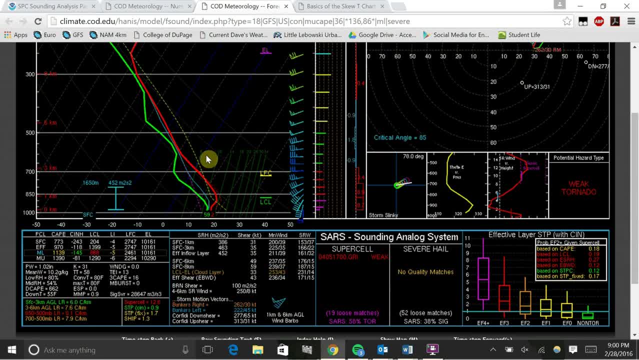 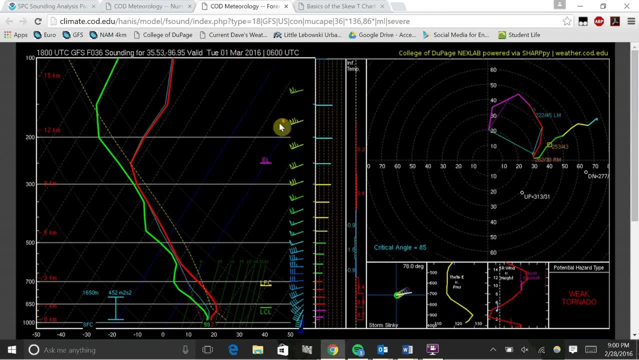 Alright, so then it's going to give you their forecasted sounding. It still gives you a timestamp here, for this is for Tuesday, March 1st, And this is called a forecasted sounding. Now a word of warning about forecasted soundings. 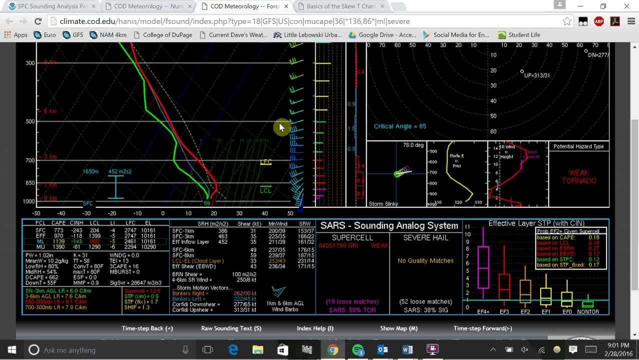 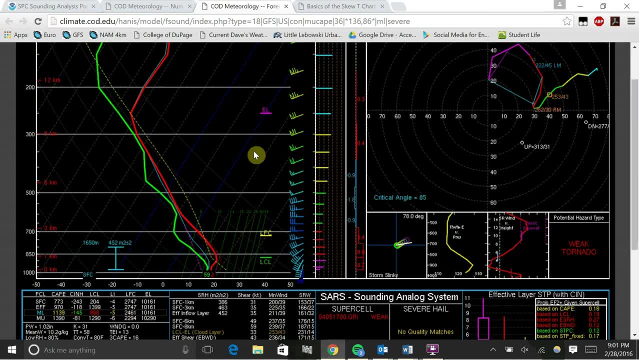 A lot of usefulness in a SCU-T is really seeing the small details of the temperature profile of the atmosphere. So if you're going to use a forecasted SCU-T, try not to go more than 72 hours out from the current time. 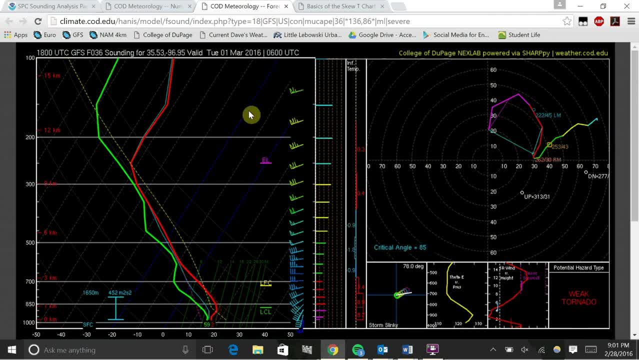 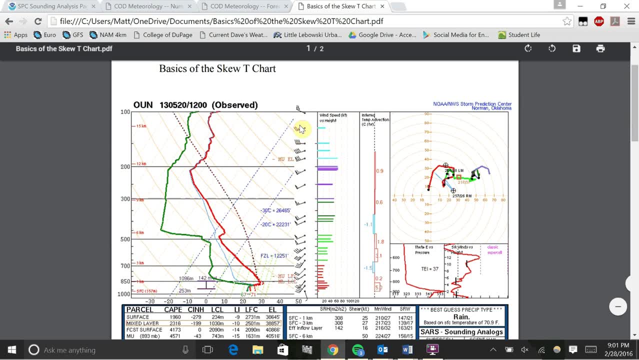 That's when models tend to start losing their good resolution. So it's a good idea to have a good reading of the temperature profile of the atmosphere. Alright, so let's talk a little bit about how to actually read a SCU-T. 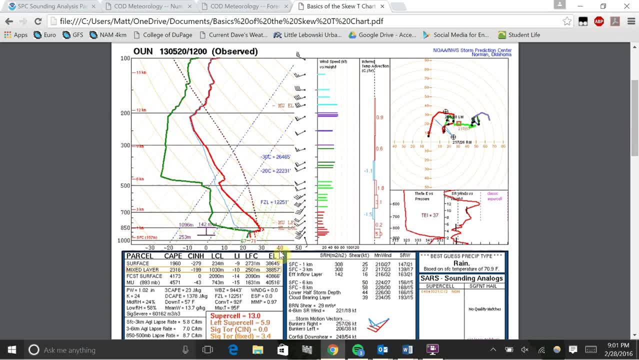 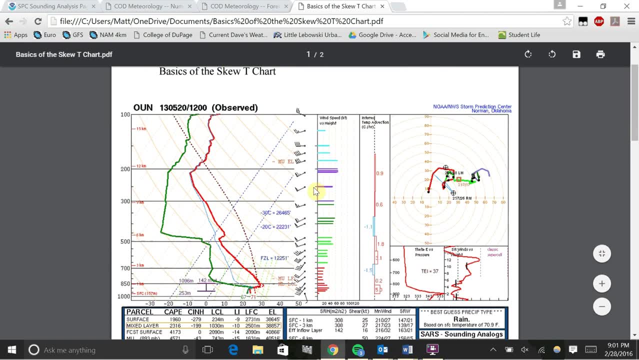 Now, the first thing that you're going to want to notice is that there's a lot of stuff going on here. This is from the SPC website. There's a lot of stuff going on here. What I want you to first focus on is this box right here. 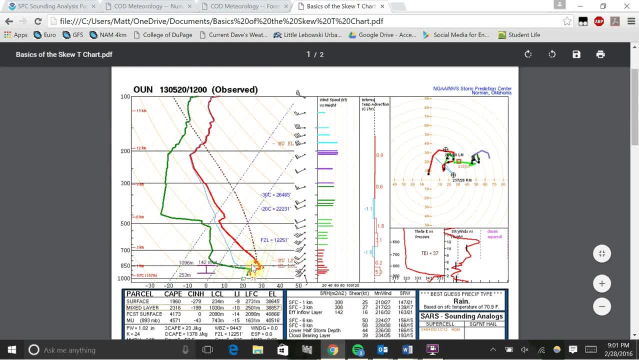 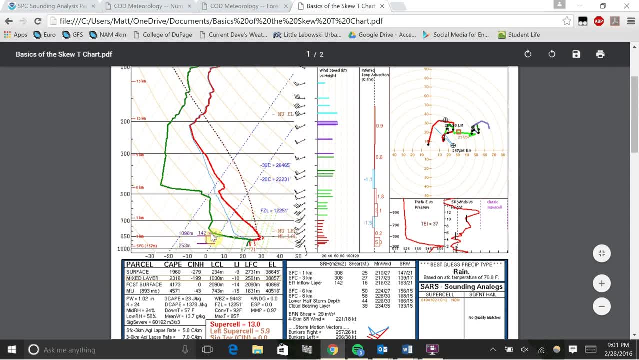 This here is the actual SCU-T. What you have here is the red line representing the temperature- This is the actual SCU-T- The green line representing dew point And the dotted line representing the path that a developing thunderstorm would take temperature-wise. 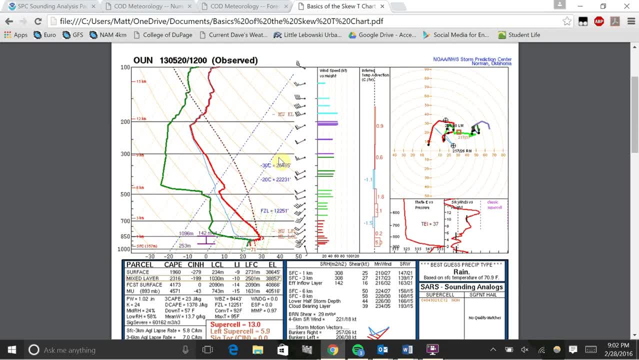 So the reason it's called a SCU-T is: you see these dotted blue lines here that are at an angle to the bottom. Those are actually the constant temperature lines. So here at the surface we've got a temperature of 71 degrees, or about 22 degrees Celsius. 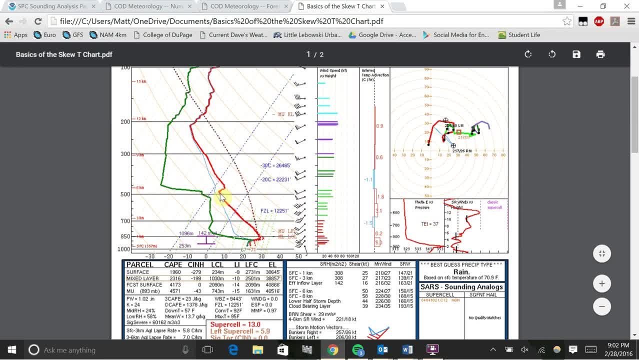 But say you go up to 500 millibars, You find where it's at And then you trace the diagonal line down And you find that the 500 millibar temperature is actually about negative 15. You don't want to go straight down? 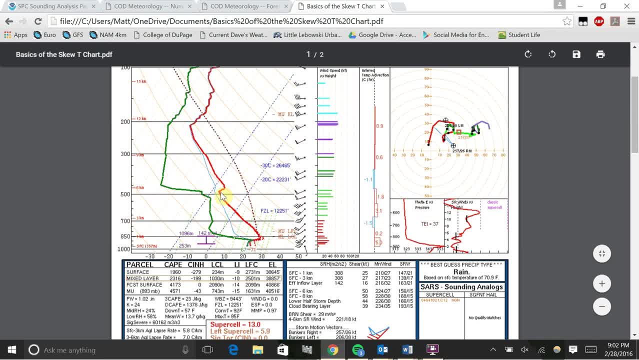 That would give you an incorrect reading. That's why it's called a SCU-T. The temperature lines are skewed, So you go down diagonally along this dashed blue line. The same angle, And it's the same thing for the dew point. 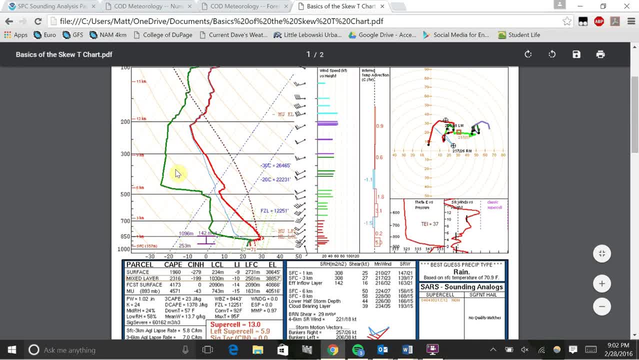 Dew point goes up And it gives you a And it gives you a good indication of how much moisture is available in the atmosphere. Coming back to the dotted dark red line, here This becomes really important in determining whether or not thunderstorms are going to actually form. 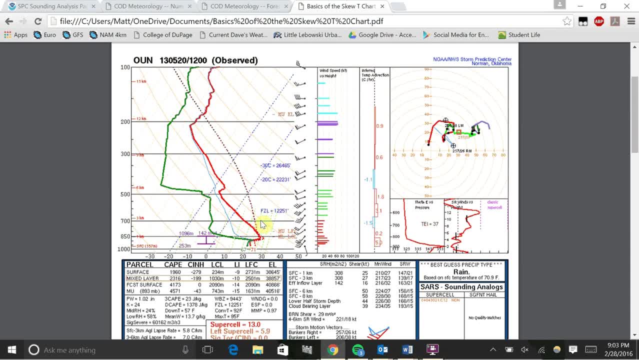 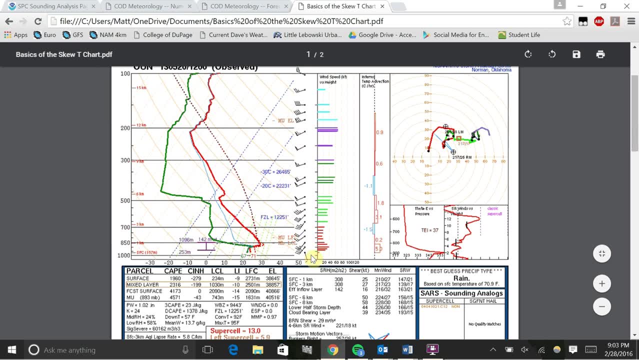 We'll get into that a bit in a little bit, But at first I want to go over some more basics here. On the right-hand side we have the winds, Typical wind barbs as you should know about from maybe an introductory meteorology class. 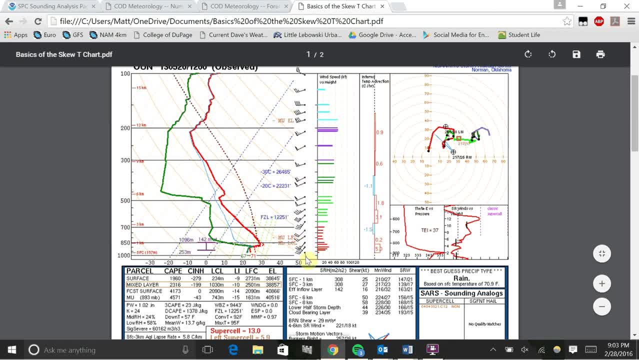 Or just looking at some other model data, But it gives you a very complete representation of the wind as it changes with height. Here you have the hodograph. Hodographs can be very useful for severe weather forecasting, Especially tornadoes, But I'm going to skip those for now. 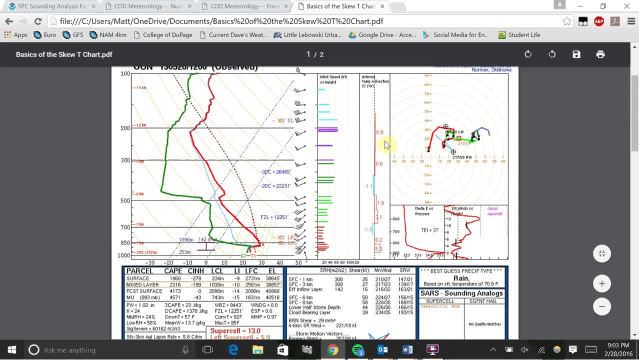 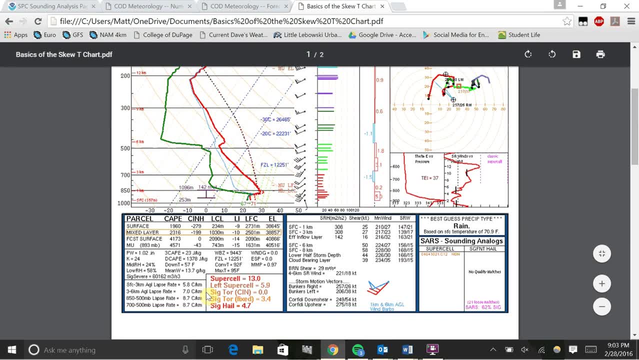 They're more advanced And basically all you need to know about winds can be found on the bar side of the SCU-T Down here. we've got some severe parameters, But I'm going to talk about those in a minute. We'll get into that in the next section. 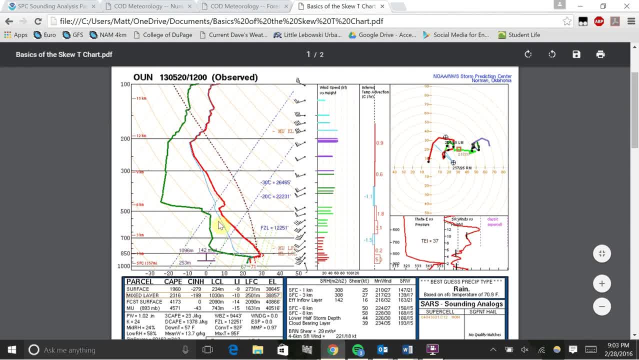 So, to recap how to read a SCU-T: You've got the vertical temperature, You have the vertical moisture And you have the parcel path, The path of temperature that a developing thunderstorm would take. Now, before we talk about, 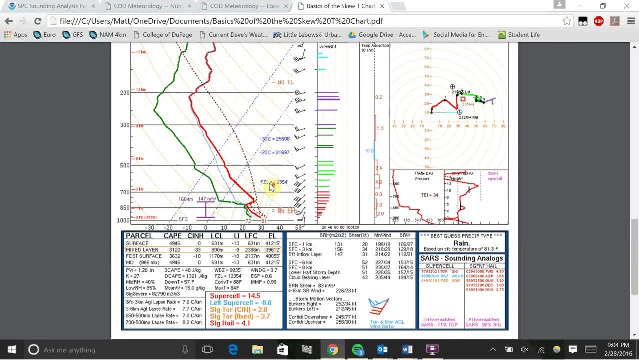 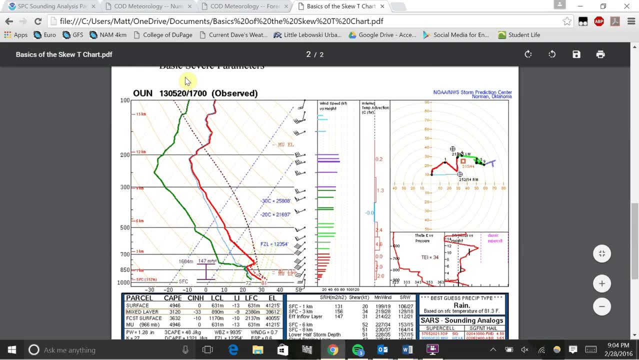 Let's just go into it, Alright, so basic severe parameters. Now, this sounding is still an observed sounding, But if you notice it's taken at the same time stamp as, Or the same day- pardon me- as the observed sound. 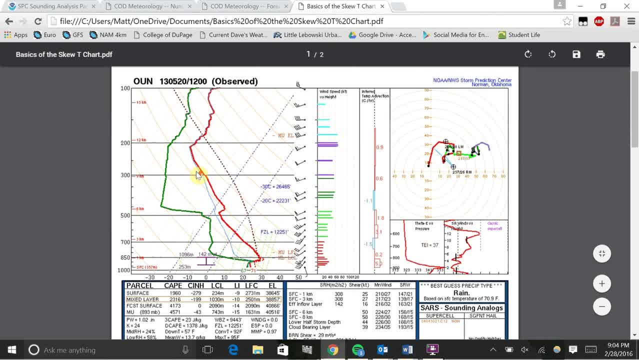 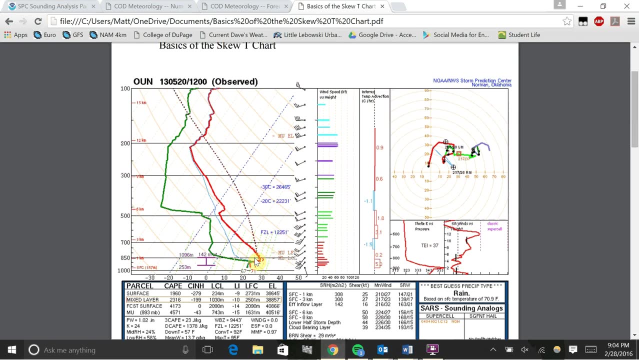 Or the first sounding. It's just five hours later. So in the first sounding you see how this dashed red line has to cut underneath. So think about what you know about buoyancy If the parcel, If the developing thunderstorm, becomes colder than its environment. 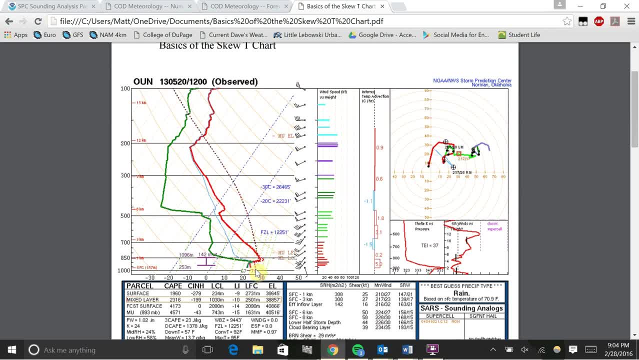 cold air. Cold air relative to the environment sinks. Warm air relative to the environment sinks. Warm air relative to the environment rises. So if it has to go through this part where it's going to be colder than the environment, a thunderstorm cannot form. 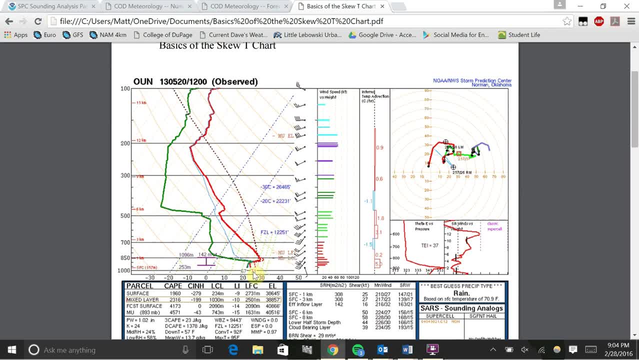 This is what we call a cap, A capping inversion. You'll see these a lot on severe days in the southern plains, Where the temperature above the surface is actually warmer than the temperature at the surface. This prevents storms from forming. And how to break the cap? 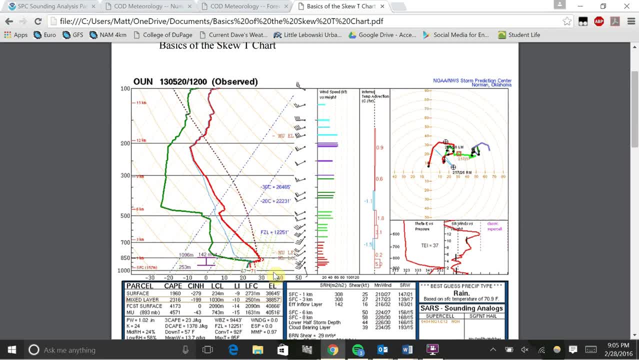 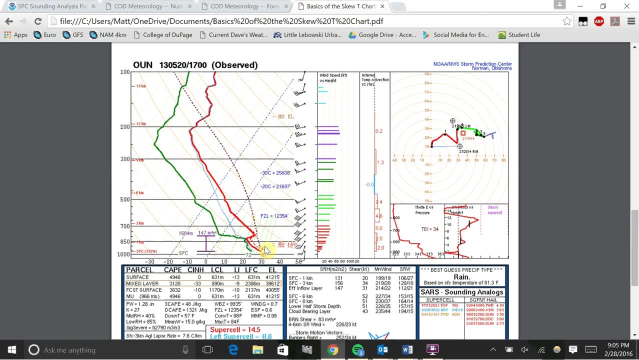 or if the cap will break, is one of the very, very key elements in severe thunderstorm forecasting. Moving down, you'll see that as the day warmed on the dashed red line no longer becomes colder on the left side than the solid red line. 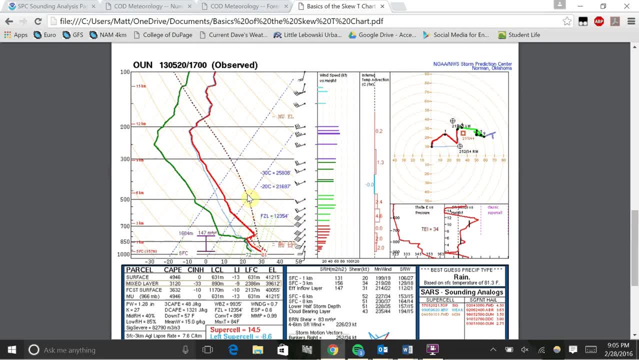 It's always warmer and warm air rises. Now the difference in temperature between the dashed red line, the parcel, the developing thunderstorm and the environment is traced out. between these two is called convective available potential energy, or CAPE. 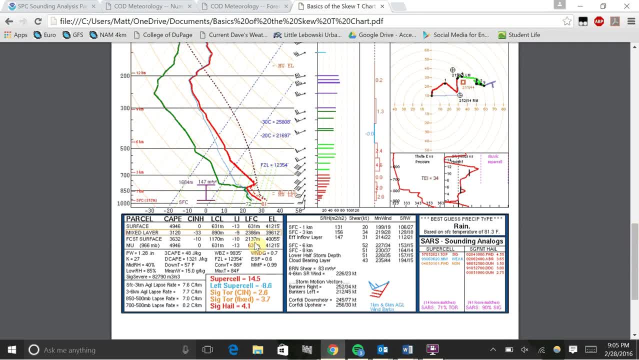 for short. Remember when we talked about the severe parameters a little bit earlier. These values here are numerical values of CAPE. So the best one to look at, I think, is either most unstable or the surface CAPE. Those will give you the most accurate representation. 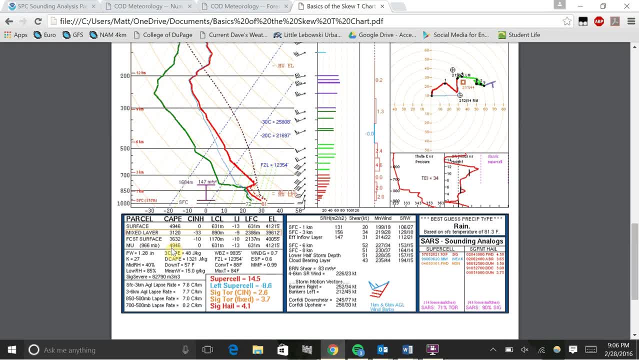 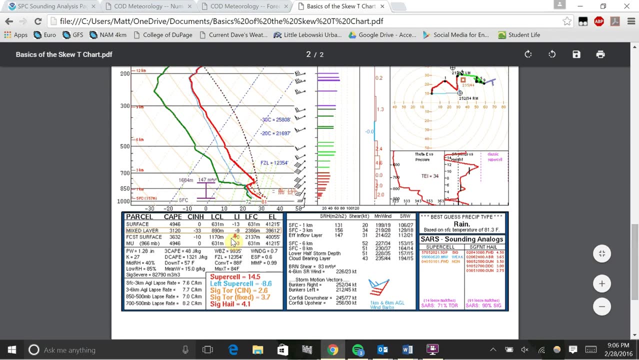 of what type of thunderstorms are available that day. You'll see here that the CAPE value is 4946.. That is absolutely incredible. I believe this is a day that many, many tornadoes occurred over Oklahoma. You only need CAPE. 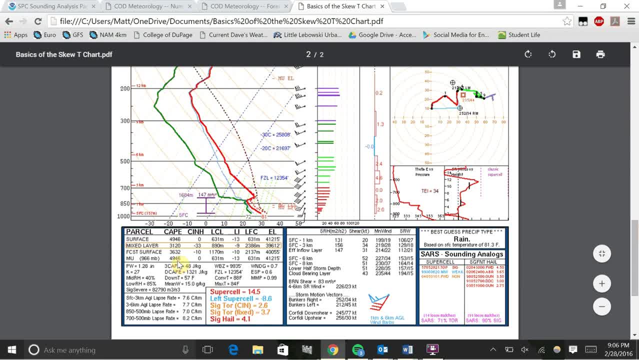 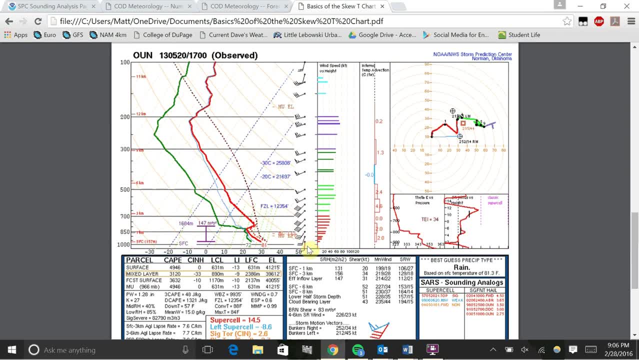 values in the 1000 to 2000 range to initiate tornadic supercells. Another big thing to look for in developing very, very intense thunderstorms is winds turning clockwise with height. You see, here we've got great winds out of the south. 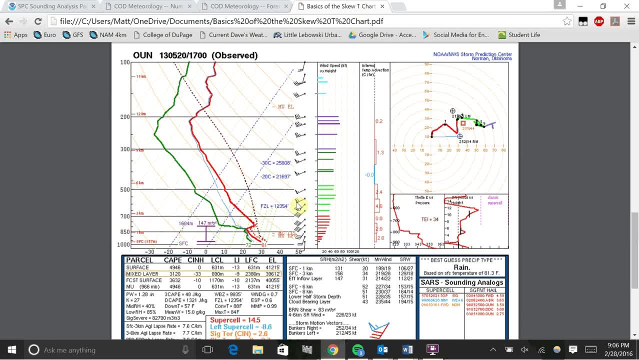 at the surface and winds almost out of the west at 500 millibars. That is just indicative that rotation is going to get developing very early and very quickly. Now back to the CAPE thing. You see how the inversion here is still. 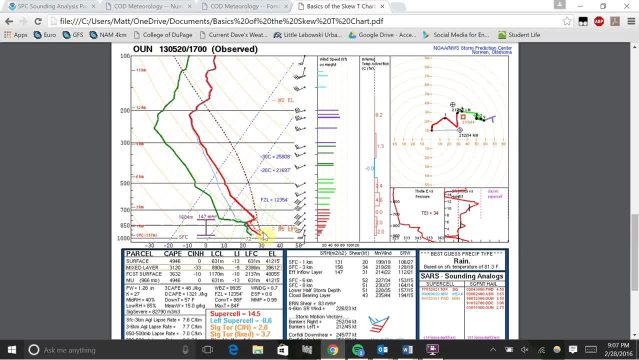 present, but the ground has warmed up to a point where the parcel doesn't have to become colder. that's an environment. We talked about that a little bit earlier. This is one mechanism for breaking the CAPE. like I said earlier, Breaking the CAPE is really just. 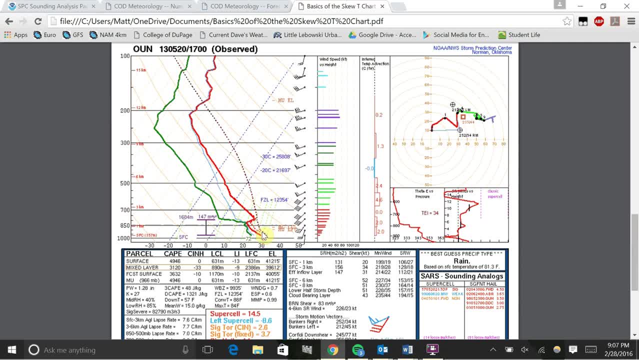 allowing the thunderstorm, or the parcel, the developing thunderstorm, to rise freely all the way to the top of its trajectory. Here is where it becomes colder than its environment again and it will sink back down. Another way you can break the CAPE is perhaps 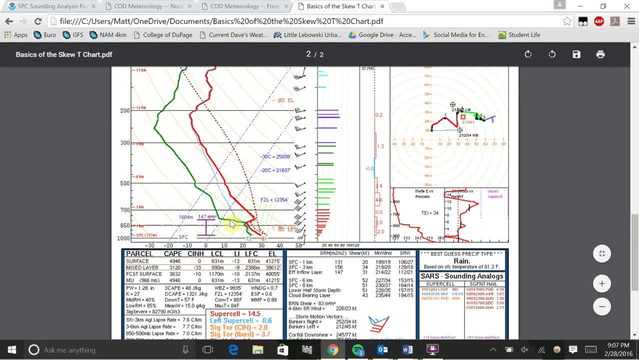 cooling off of the mid layers. If you have a deep area here, like we see here, where the dew point becomes relatively low compared to what it is in the lower layers, As a thunderstorm begins to rise, it will evaporate. and when you evaporate, 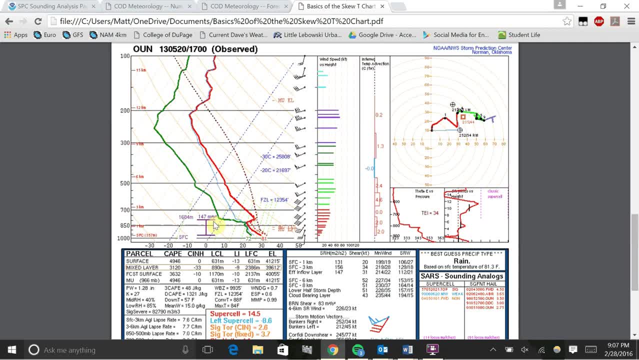 liquid water. it actually cools the environment. So that's another thing you can look for is a pronounced dry layer in the 700 to 850 range. That will also help break the CAPE. So in conclusion, we talked a little bit about 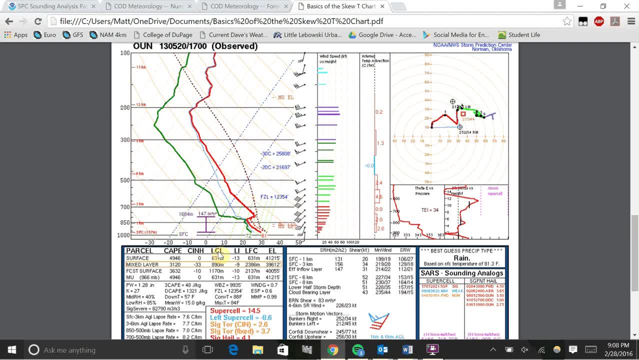 how to read a SCU-T. I gave you some instructions on that and then I gave you some basic, severe parameters to look for. A lot of CAPE, a lot of area between the dashed red parcel line, developing thunderstorm line and the temperature line, And every. 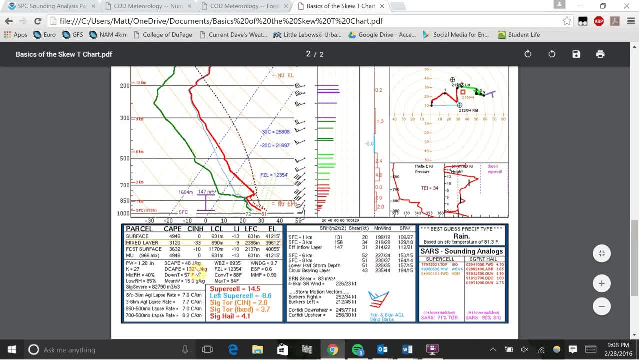 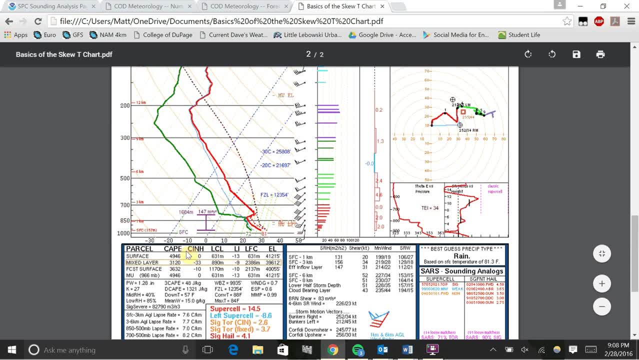 sounding is going to have all of these components. We talked a little bit about the numerical values. Oh yeah, SIN here this is pretty much a measure of the CAPE: how strong the CAPE is Here you see at the surface, and 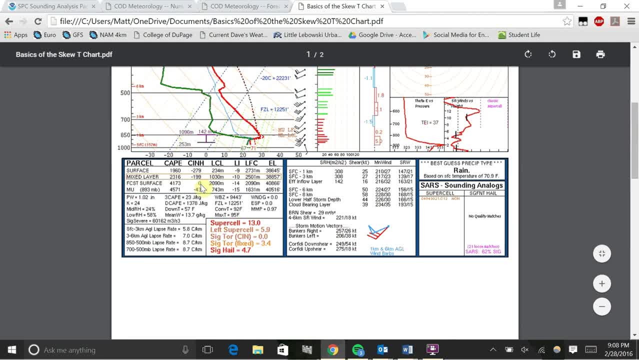 most unstable. it's zero, so you don't need to worry about it here. But up here at the beginning you have a negative 199.. That is a big number that's going to inhibit. So you see, the forecast surface is zero, so it's forecasted. 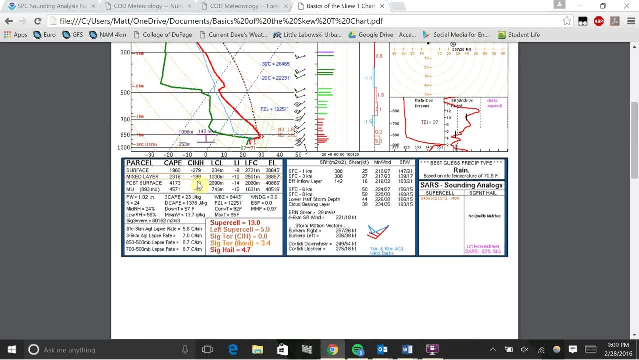 to break the CAPE. But in the morning there was quite a bit of SIN keeping the storms down. So if you see SIN in the negative 50 to negative 200 range, it's going to be hard to develop thunderstorms at the current time. But if you can, 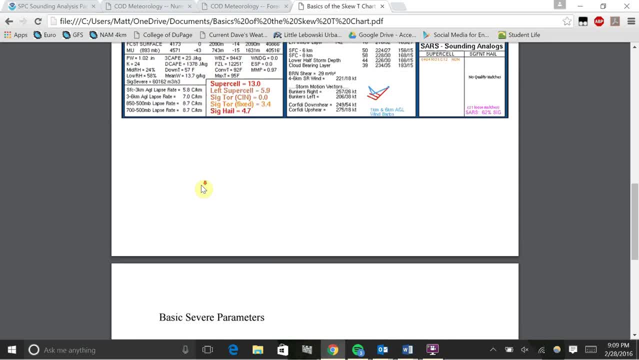 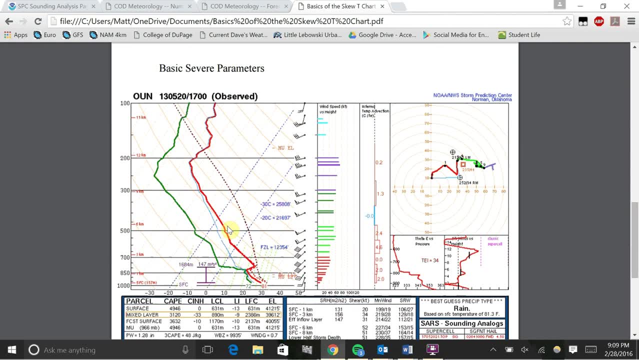 forecast it. that's when you can see things starting to get interesting. So, in general, SQTs can be very, very simple and very, very useful In the future. I hope that you're able to use these a little bit better. 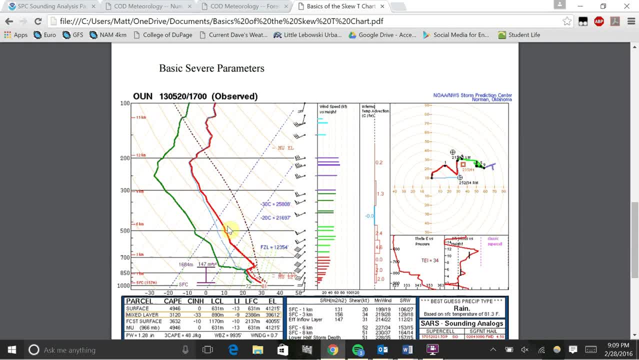 than maybe you have been in the past, Or I hope you're able to find them and start using them in your amateur weather forecasting or anything else that you might be trying to do with weather. They're also really useful for flying in the winter with freezing. 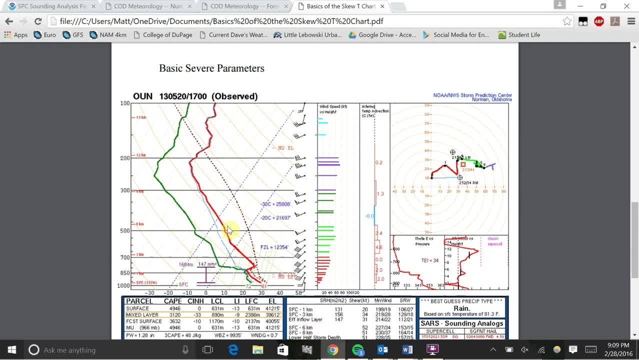 levels, but that's a whole other story. So for the time being, I hope you enjoyed this presentation And if you have any questions, never hesitate to contact me. I would love to explain SQTs more in depth to you. Hope you have a great day. 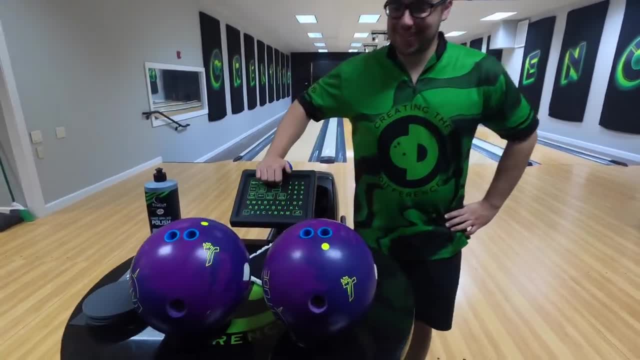 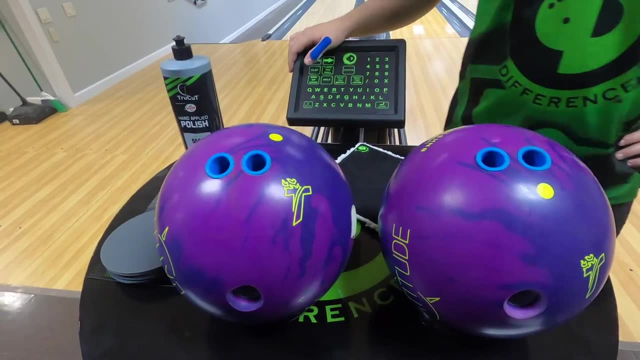 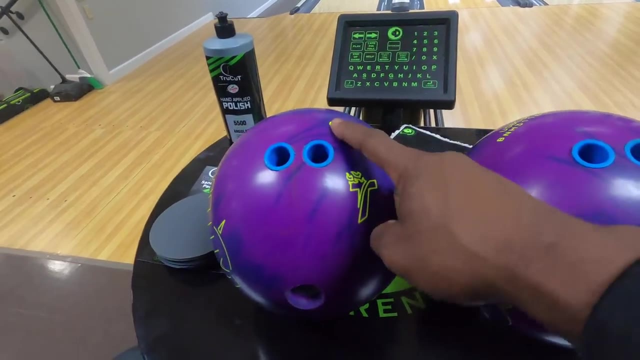 CEO Roderick from Create the Difference. We're going to talk to you today about pin up versus pin down. Now what we've done is we've actually only changed the pin up to pin down, second angle of these layouts. So the pin to positive axis point is the exact same distance which happens. 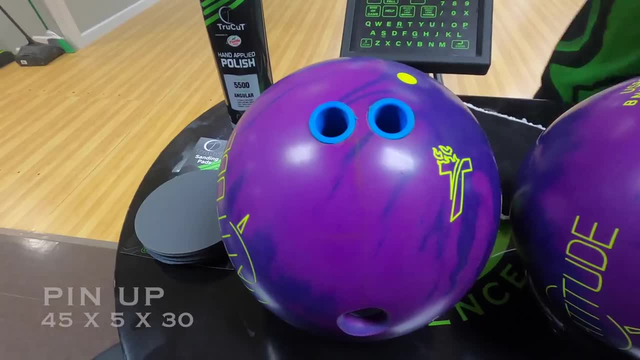 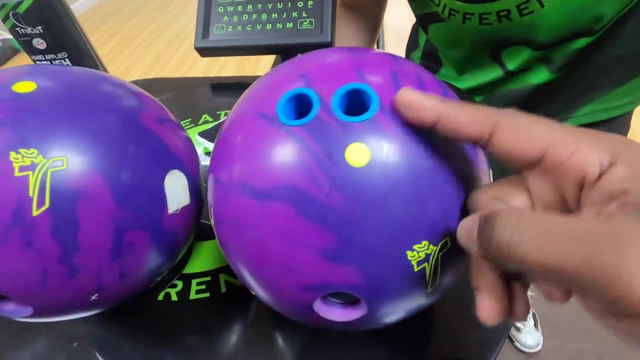 to be five inches, And the layouts on both these balls. this ball right here, the pin up ball, is actually 45 by five by 30. And the pin down ball is 45 by five by 75.. So the 75 is what's making it. 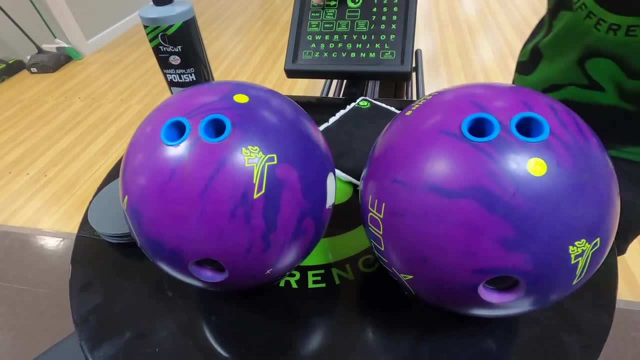 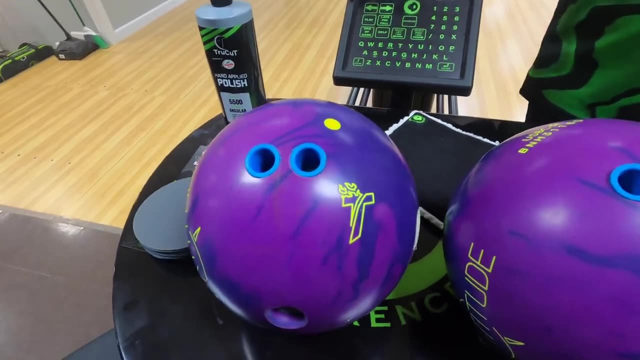 pin down. The 30 is what's making it pin up. That's the only difference between these two bowling balls. We didn't move the pin around because if we did, we'd have two variables to try to understand instead of just one. So this is a pin up ball. That's at five inches away.